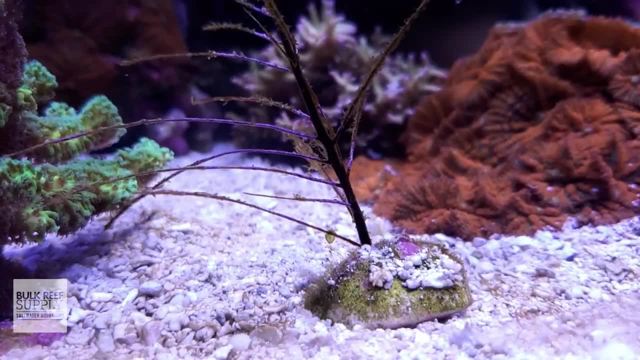 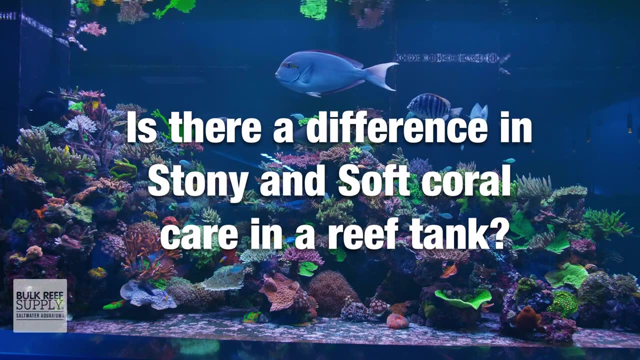 of stony corals. their skeletons are usually dark, brown or black, super thin and very bendy. So the next big question: is there a difference in stony and soft coral care in a reef tank? Yes, there absolutely is a difference. 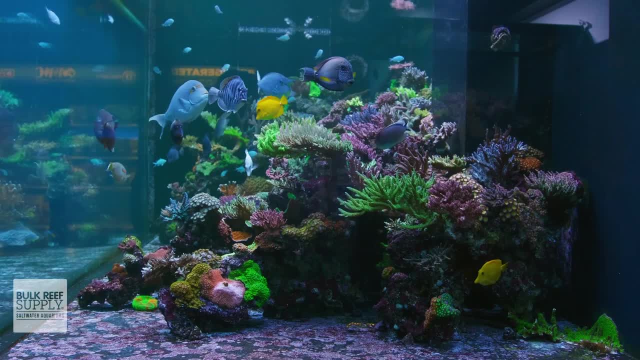 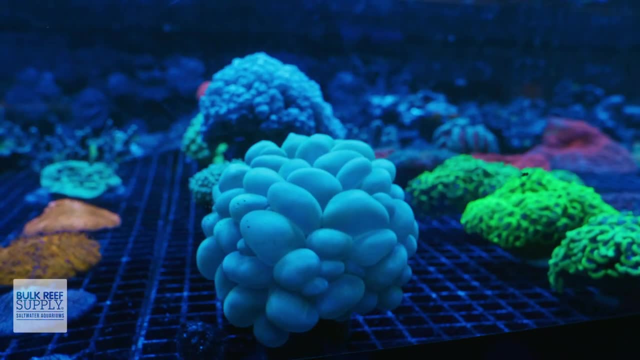 And when it comes to caring for corals in a reef tank, stony corals tend to be more demanding than soft corals, especially for those who are newer to the hobby, Because they don't have a true skeleton, soft corals tend to be much less demanding. 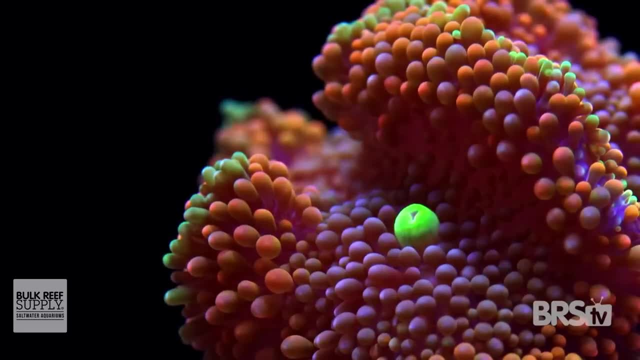 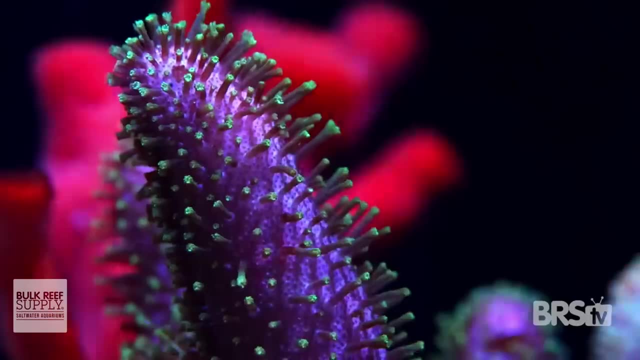 of alkalinity and calcium. Soft corals also tend to come from nutrient rich environments that are silty and murky. So many soft corals have no problem in a reef aquarium that has high nutrients and isn't dosed very often. In other words, they're very hardy. and usually do just fine in an aquarium with less than ideal conditions for stony corals. They're also typically less demanding of intense lighting as well, So you can easily keep them without getting high end light fixtures, With, that being said, having a good reef light. 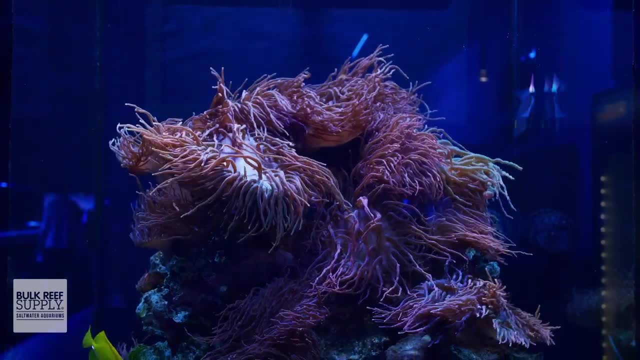 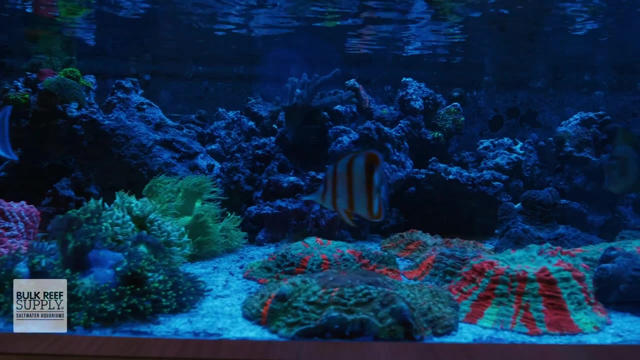 is going to have a pretty large impact on how colorful many of those soft corals will be. LPS, or large polyp stony corals, are a great place to start for reefers that want to get into stony corals, While they will definitely require you to test your aquarium. 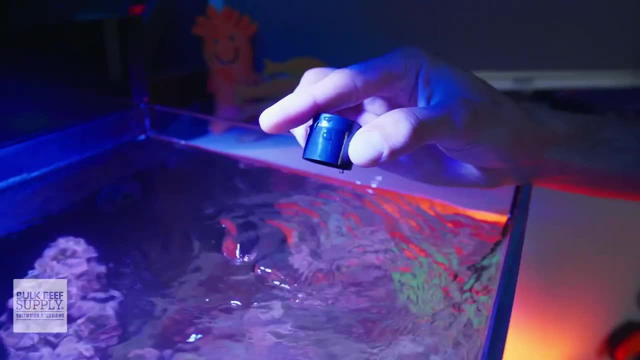 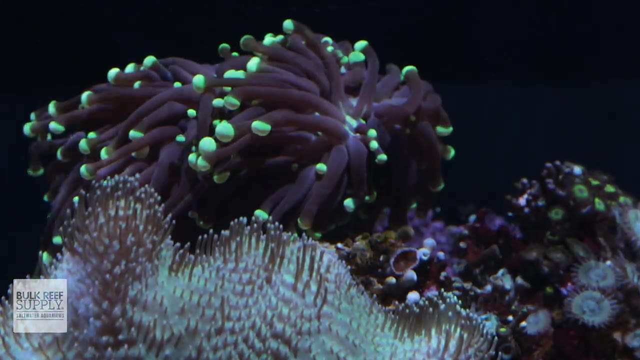 at least weekly, and dose additives to maintain the levels of two major elements, alkalinity and calcium. many LPS do appreciate higher nutrients, just like soft corals, and do just fine with similar light conditions. LPS, however, can also benefit quite a lot from proper flow. 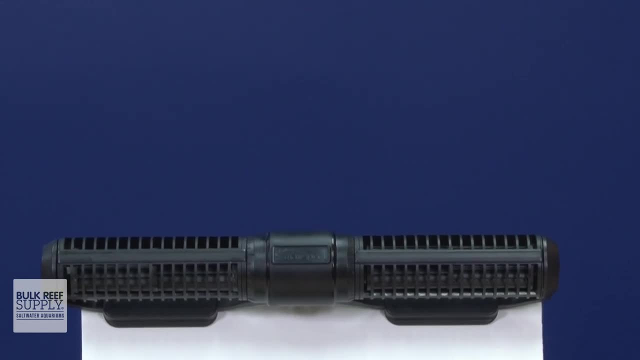 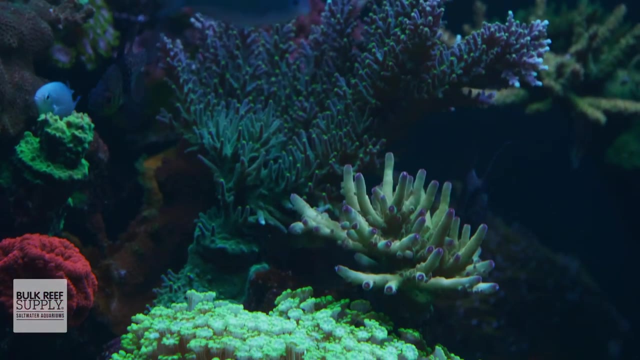 so making sure you have a capable wave pump or pumps is also going to be important Now. SPS, or small polyp stony corals, are considered to be the most difficult corals to keep. They are the most sensitive to water parameters. 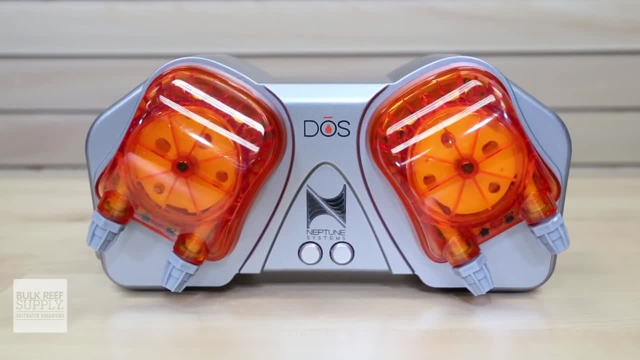 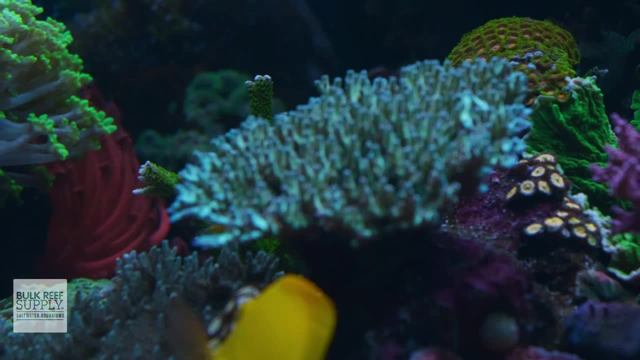 require stable conditions with optimal levels of not only the major elements, but also minor and trace elements. Many of them, especially Acropora, require pristine water with just the right level of nutrients. in order to thrive and look their best, They typically require the most intense lighting. 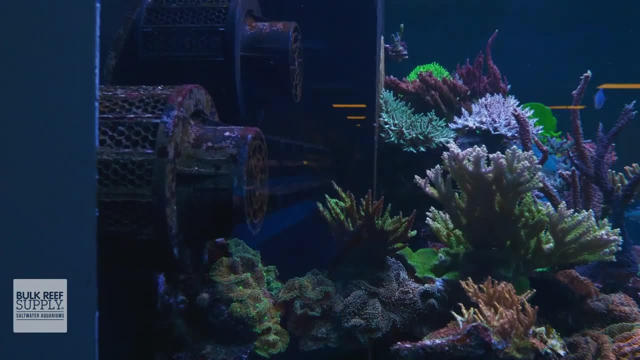 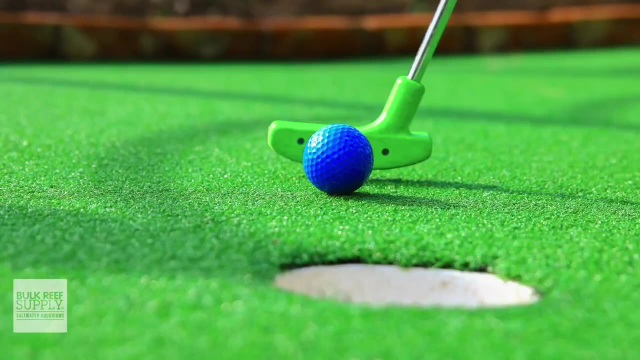 along with the most intense and thoughtfully implemented flow. An aquarium designed for SPS corals is going to be the most challenging and often the most costly in equipment and additives. If a soft coral reef is mini-punt, an SPS reef is the peak of professional golf. 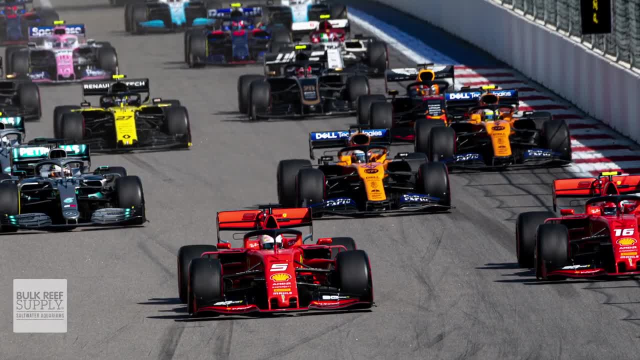 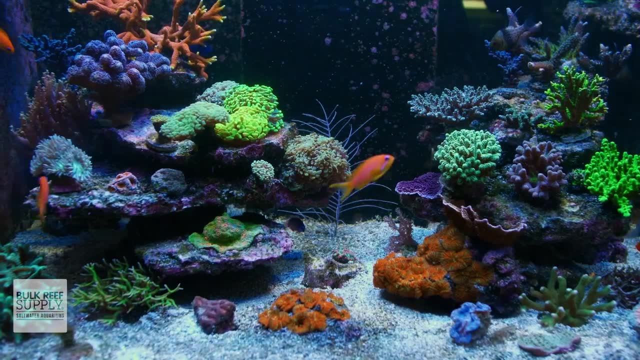 If a soft coral reef is go-karting, an SPS reef is Formula One. If a soft coral reef is, I'm sure you've got the idea. But what about mixed reef tanks? Mixed reefs are the ones that have a little bit.